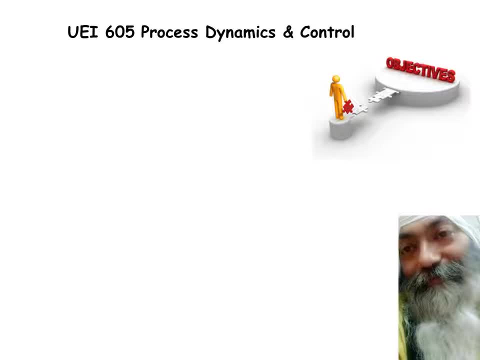 using this code every place, and we want to make it very clear right in the beginning that in whatsoever kind of interaction we have, either through zoom meetings or face-to-face interactions, as the case may be- we shall be having maximum interaction through whatsoever means. That is, it's a two-flow communication, two-way communication and the flow of information. 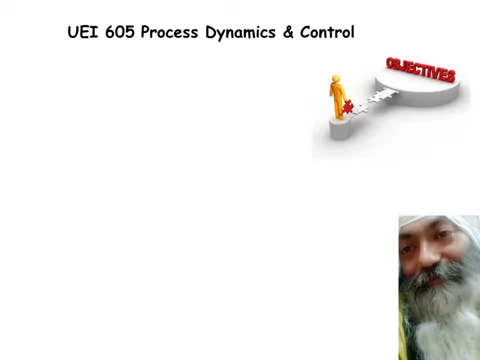 shall take place from me to you and you to me. So it's very clear what shall be the objectives of this course, Like: why do you want to go in for this course? Because this course is to make the students understand basic ideas, the challenges, techniques and applications. 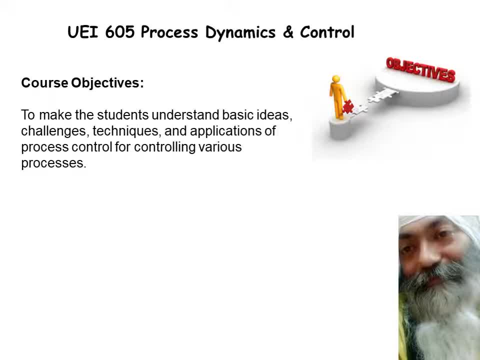 of process control for various processes. So normally these are the chemical processes. and once you say it's a chemical process, don't get scared, it's got nothing to do with chemistry. We will not be dealing any chemical equations over here, but once you go in- for if you look- 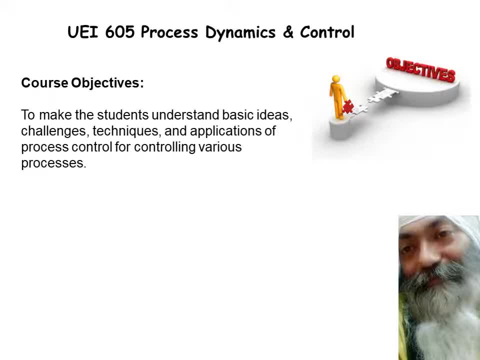 around any kind of process with some chemical reactions taking place. even making of chapati is a chemical reaction. So that way, if you see, you have paper and pulp, thermal plants, cement industry, for example, You have chloralkali, You have fertilizers. 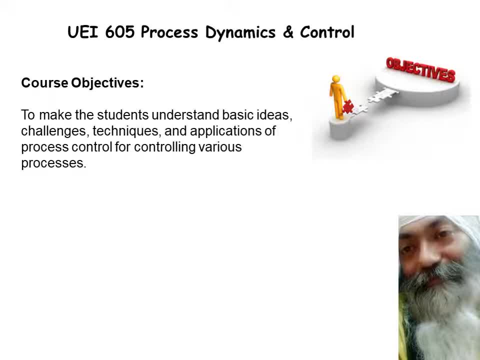 You have refineries and so on and so forth. Everything, every process. most of them are involving some kind of chemical process that needs to be controlled and in order to control it, you must know the behavior of the process or the dynamics of the process, how the process is going to behave with respect to time, how 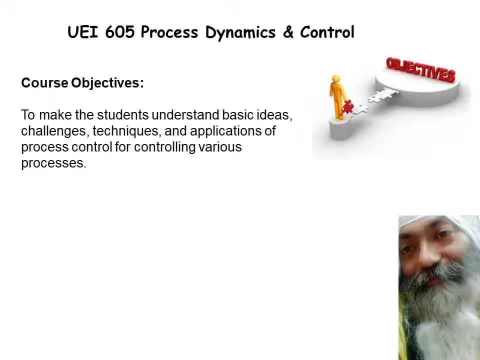 to control it, how many seconds the process takes and see how many minutes the process �� then how the process is going to move from certain cycle depending upon the activity of this process on specific월 Hs if you see what you see there are going to be six steps. 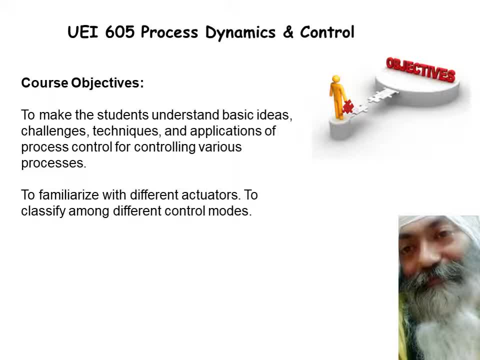 Uh, or you may have to remember just one stepеше, for example the ring codes and all the steps that are in order that we can control regulars in this course and tych hents under different conditions. so we shall be studying all these things in this course and the objectivists. to familiarize the students with different actuators, to classify amongst the different control modes. but these are the basic objectives of this course. Hes given us a slot of three lectures and just send out a summary of all the tasks that we have completed so far. 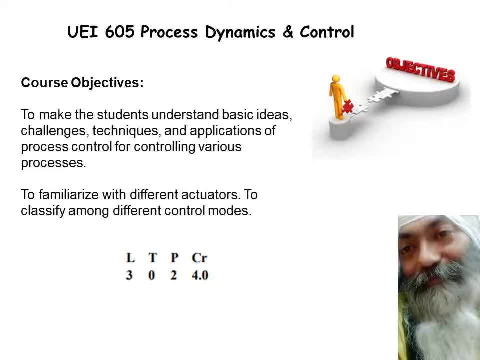 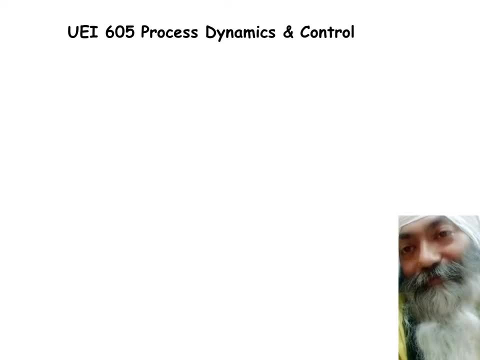 Hes and two hours practicals in, or the lab work as we call it, in one week. Now going in for the syllabus which I'll be dealing with, the introduction part, the historical perspectives, incentives of the process, control, synthesis of the control system and classification. 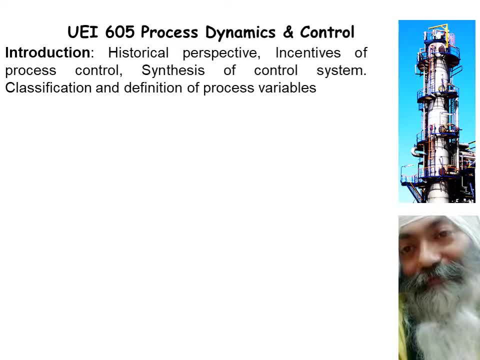 definition of process variables. and here, you see, is one part of the chemical process, just to give you an idea how the process plant looks like and what are the various components of this process plant and how do they behave? that's what we're going to model them. So we have to have a proper 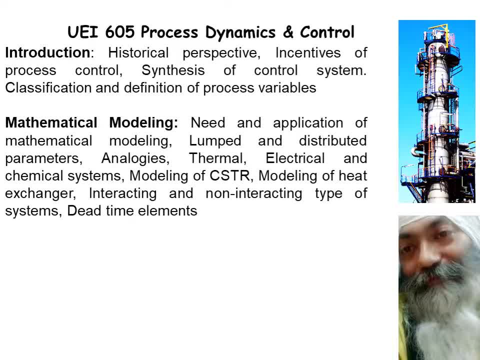 mathematical model and it can be a lumped model or a distributed model and I will not go into the details Right now. but we have to take into account the various aspects: analogies, thermal, electrical, chemical modeling of CSTR, as you might be knowing in detail what it is, heat exchangers, some of the 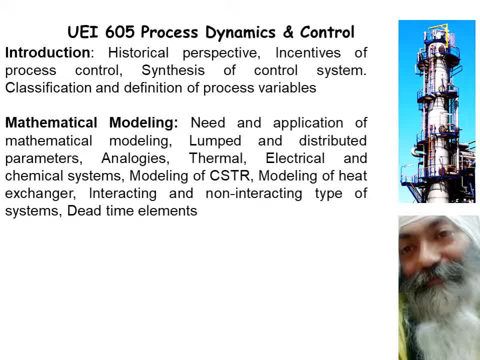 interacting and non-interacting time type of systems, the dead time elements. don't get scared by these words. these are very wordy Things as such, but as and when, slowly and gradually, systematically, I shall be introducing you the concepts in the form of mathematical equations as well, and its applications, because 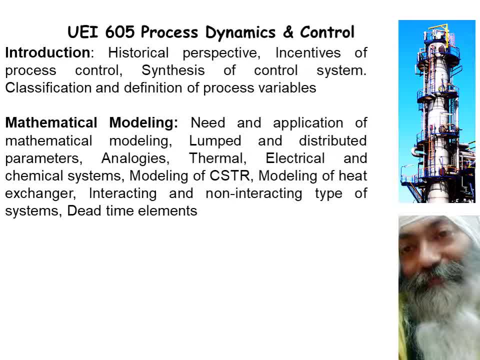 of my experience in the industry for last so many years. I've been working with the industry directly for seven and a half years, and indirectly- I don't know how many number of years I'm working as a consultant. so I will be giving you the application of 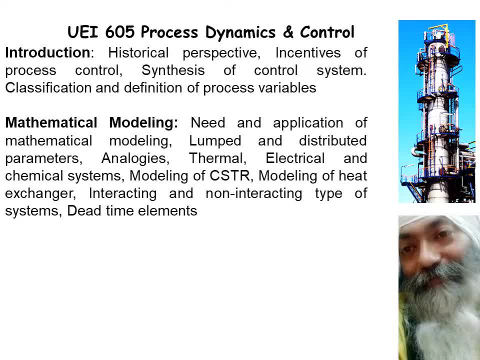 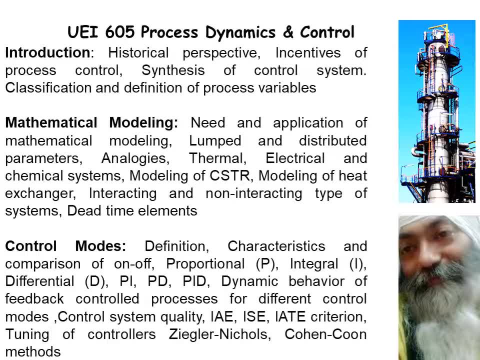 all these models in various process plants control these process. you have different modes. you might be aware of PID, so I shall be giving you a good kind of dose, you can say, of these PI, PD, PID kind of controllers, where they are to be used, how the control quality is to be. 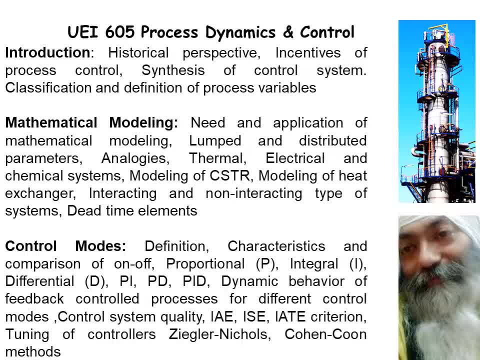 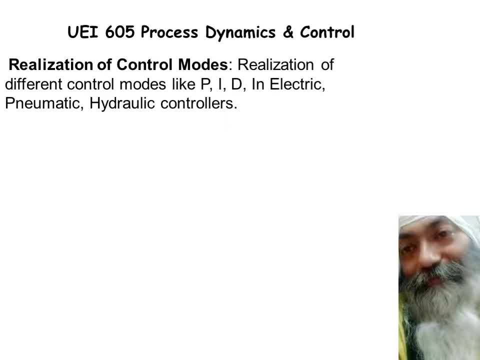 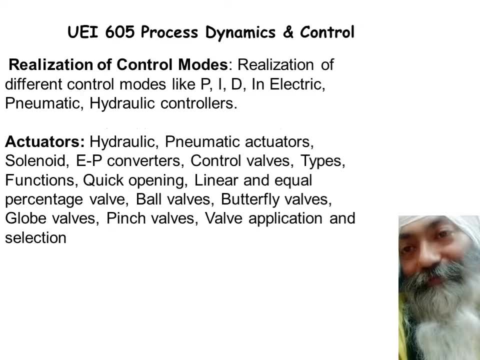 ascertained and how they need to be tuned by different methods. coming to the remaining part of the syllabus, which consists of realizing these control modes in electrical, pneumatic or hydraulic systems, we need some actuators in terms of different types of E to P converters or different type of 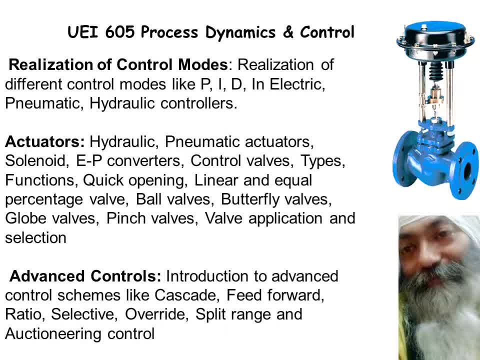 walls. and finally we have some advanced controls. a glimpse of it in the next lecture, although much of the advanced controls are taught or exposed to in another course, which probably I may be teaching or someone else may be teaching- that's by the name advanced process control. but 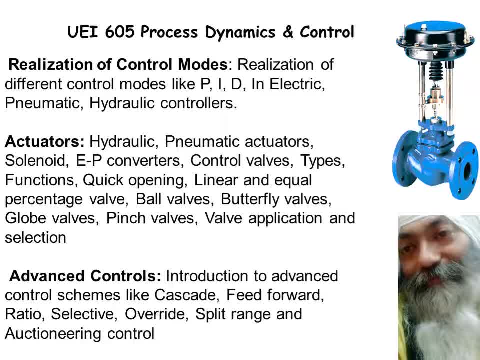 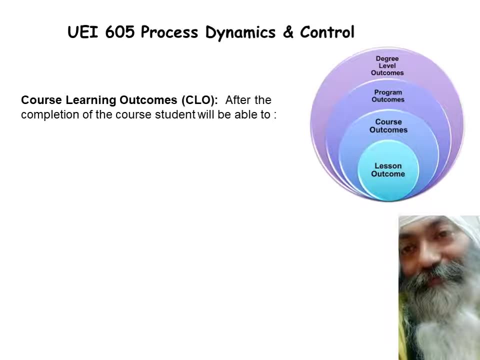 little bit of flavor of that is given in this beginning, with little bit of overlap, so as to maintain the continuity between this course and the next course. so those advanced controls like feed forward ratio and the other controls will be given in the next lecture. Finally, at the end of the course you have course outcomes. you shall be able to demonstrate the 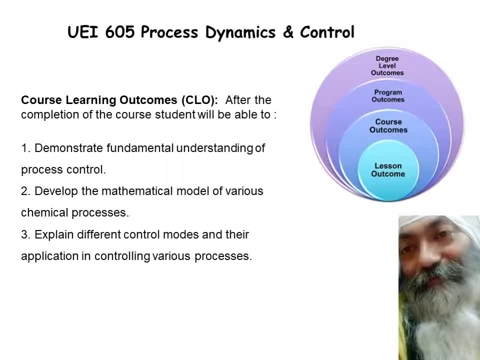 fundamental understanding of what the process control is, what the mathematical models are, what are the different control modes, how the working of electrical, hydraulic or pneumatic controllers takes place, and application of different types of actuators and control valves. so, as such, you will get a fairly cool idea of what the process control. 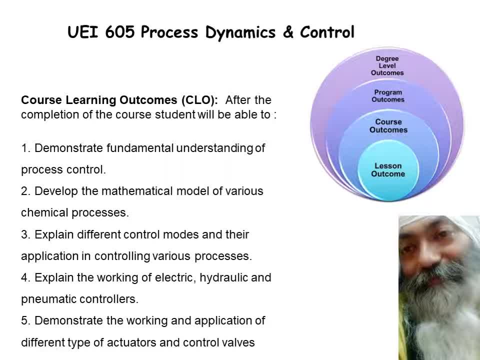 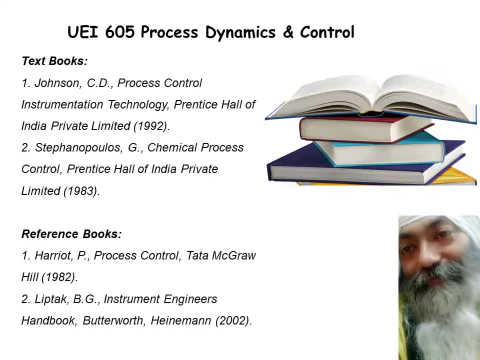 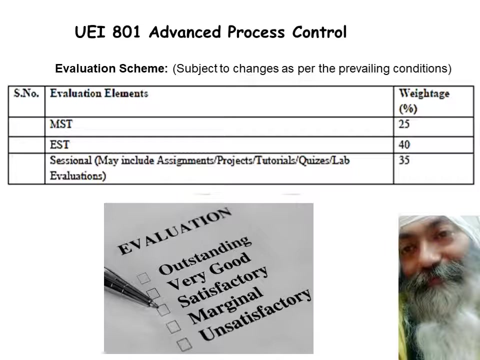 and the process plant is both in physical terms as well as in mathematical terms. these are some of the books which you shall be dealing with in the textbook form and the reference book forms. the course evaluation takes place depending upon the conditions. this is not a very hard.